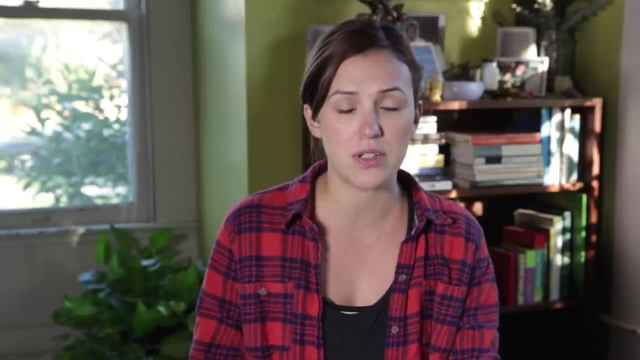 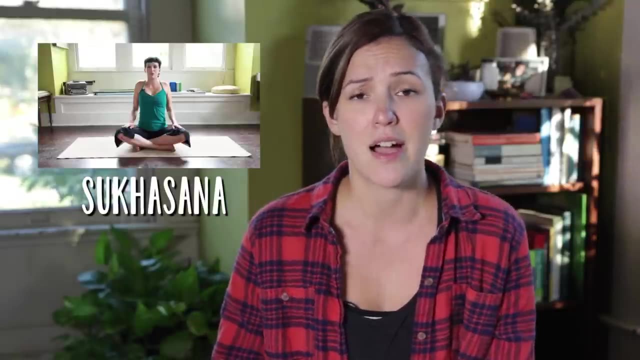 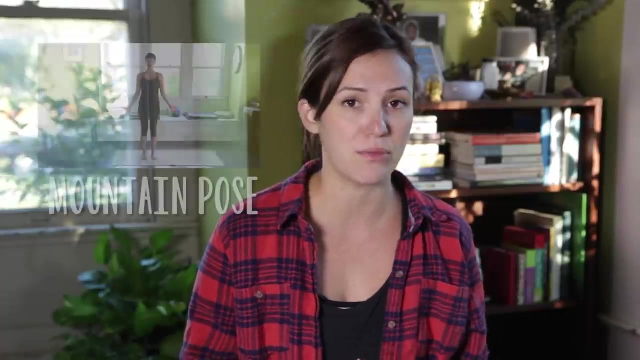 we have some great postures on the Foundations of Yoga series To get really specific. start with, actually like the first pose we ever did, which is called Sukhasana, or the easy pose, Start there. Another one I would recommend checking out is Tadasana, or the Mountain. 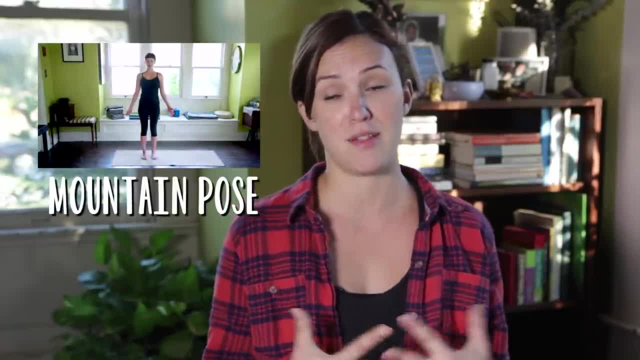 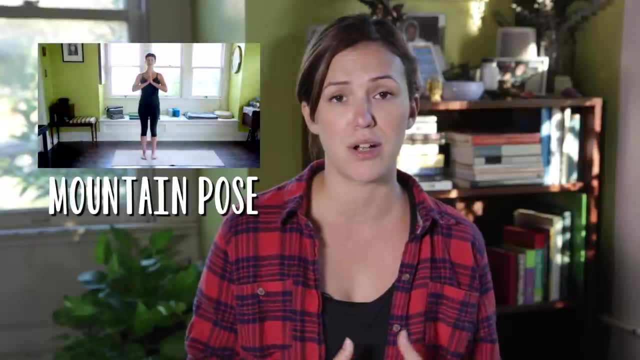 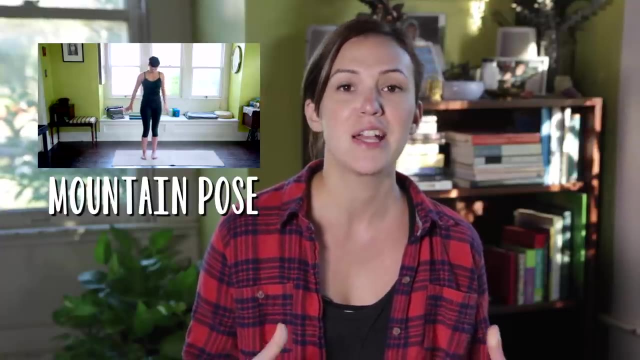 Pose. This is a posture that I, in my opinion, think will change your life, whether you go to yoga class or not. Just learning this posture and gaining full body awareness, I think, is worth the price of this video, which is free, so I don't know what that means, but it's definitely worth. 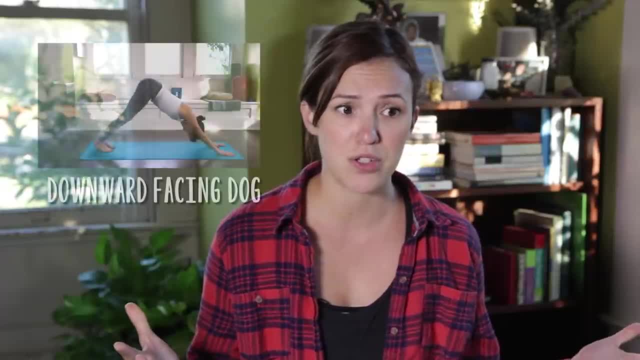 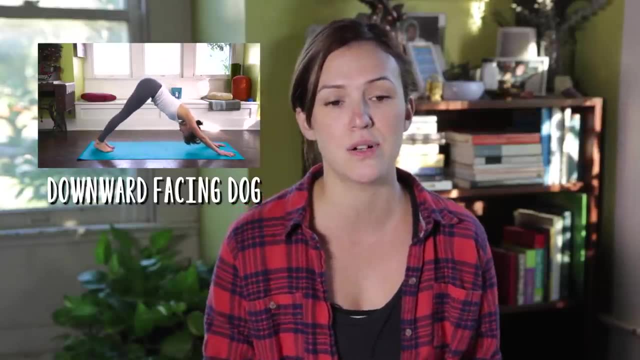 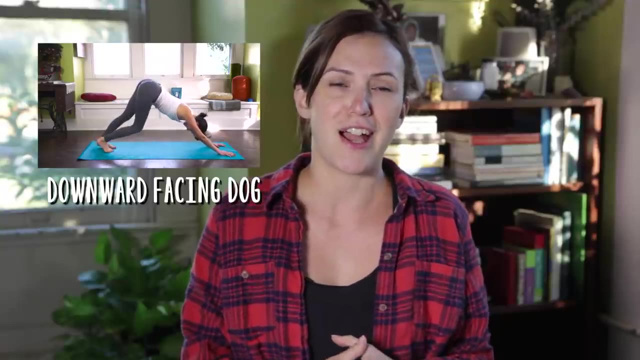 it. Another one is Downward Dog. We all know this posture. We associate yoga, Hatha yoga, with Downward Dog. but it can be a beep, You know it can. So take time with the Foundations of Yoga. Take the Foundations of Yoga video with Downward Dog and grow that posture. I think I've said 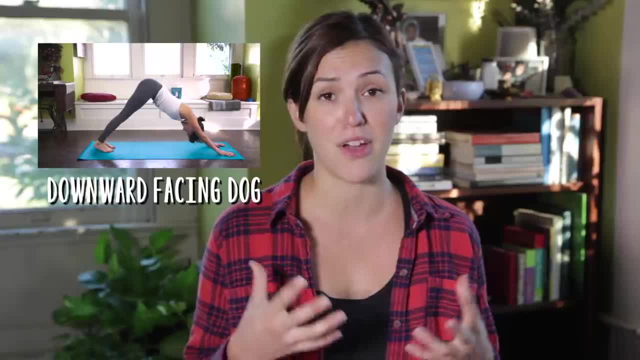 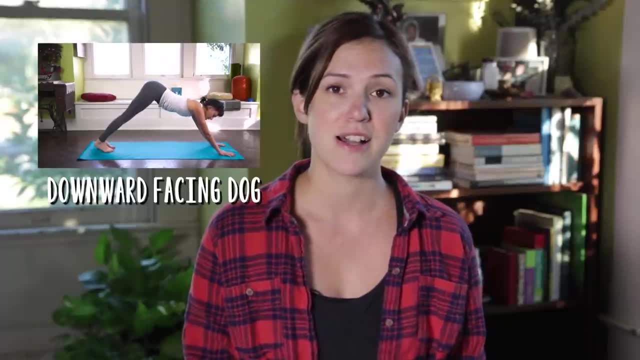 this before on the channel, but I really fell in love with Hatha yoga, with Asana the day. I fell in love with Downward Dog, and that was not right away. It took a lot of practice. so take it or leave it, whatever that means for you. 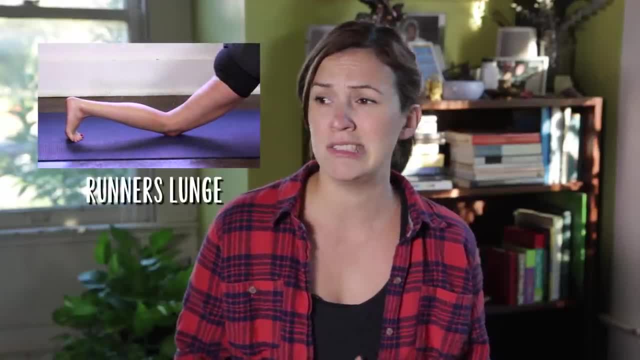 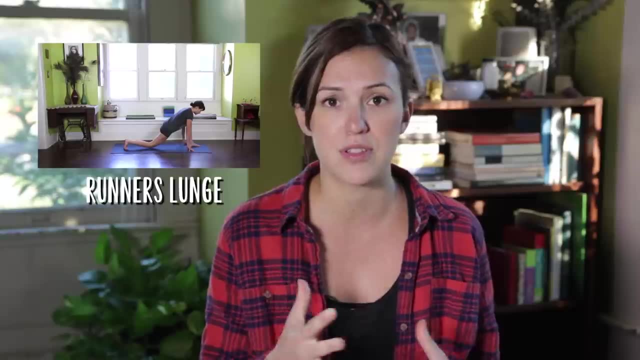 And then Runner's Lunge. I have a lot of friends, particularly men, just do not like this posture, but it is like in my top kind of What am I mentioning? Three, four, five, six, seven, eight poses to tackle as a beginner, because you will notice it grow fast if you stick. 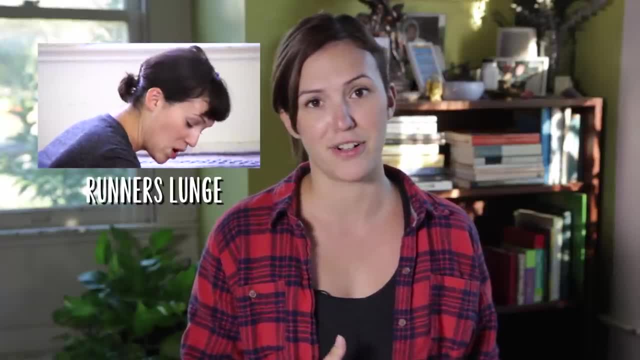 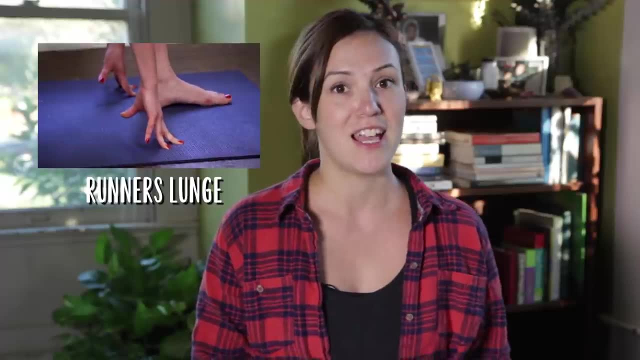 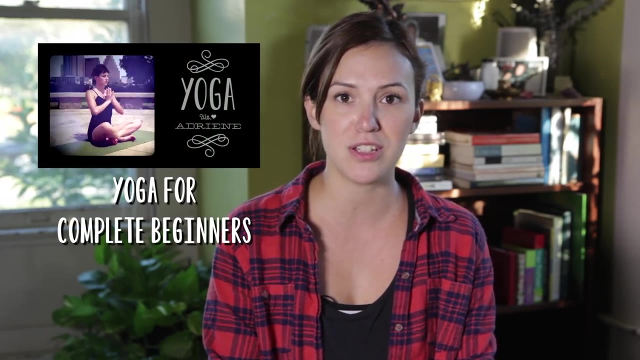 to the practice And also it's just very common in regular Hatha yoga class. If you want to go to public classes, prepare yourself for class by spending some time with me and the Yoga With Adriene channel. Another cool thing that I can add to this: where do I start? thing is we just rolled out. 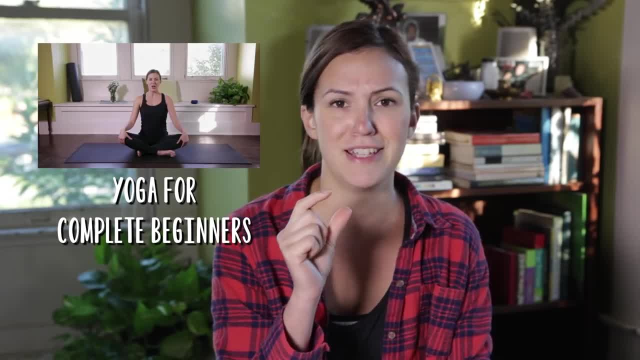 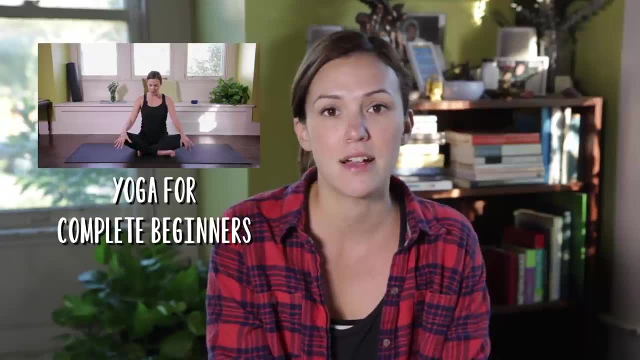 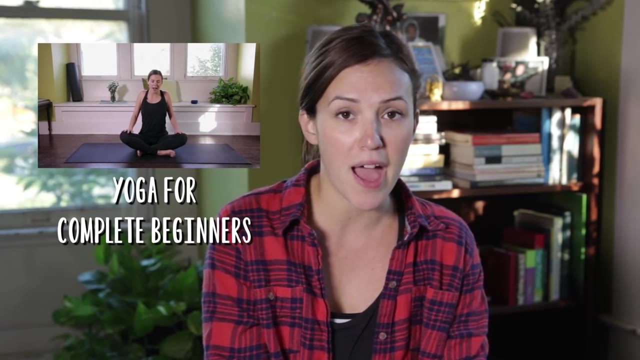 a beginner's video and it's a quick sequence. that's rather simple. It might not be easy for you right away, but it's simple, just allowing you to get on the mat without too much pressure. too many yoga pretzel poses without a whole lot of talking from me You. 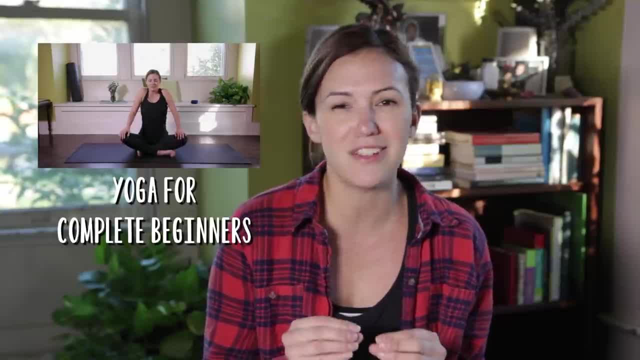 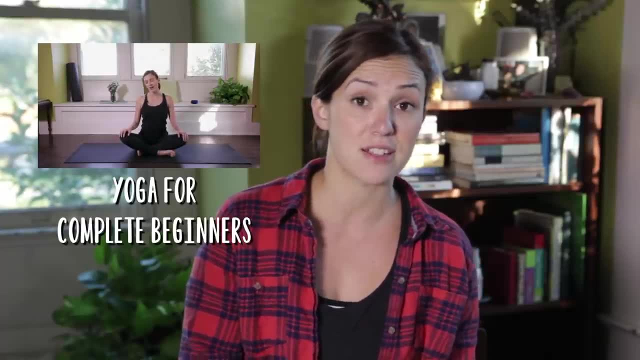 can get that in the Foundations of Yoga series, but just to give you a little taste of the experience. So check out that Yoga for the Complete Beginner and you can tackle that as a complete beginner or maybe someone returning to the practice. Maybe challenge yourself to practicing. 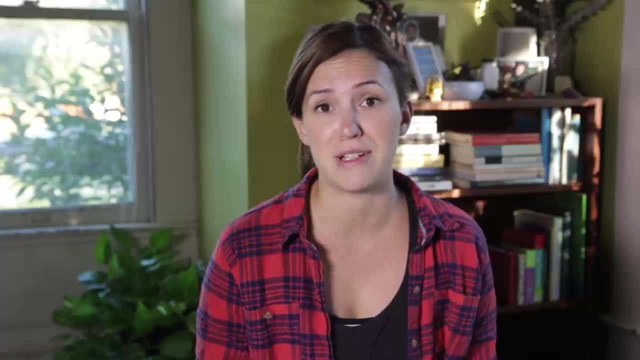 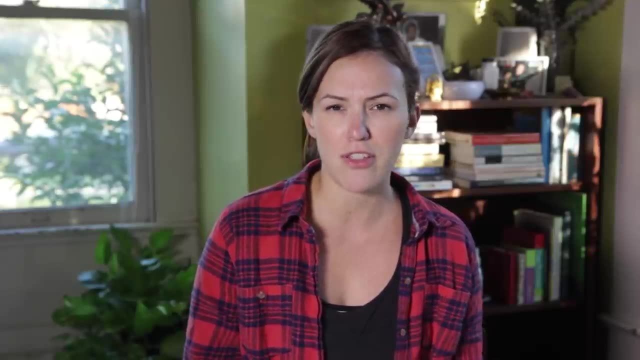 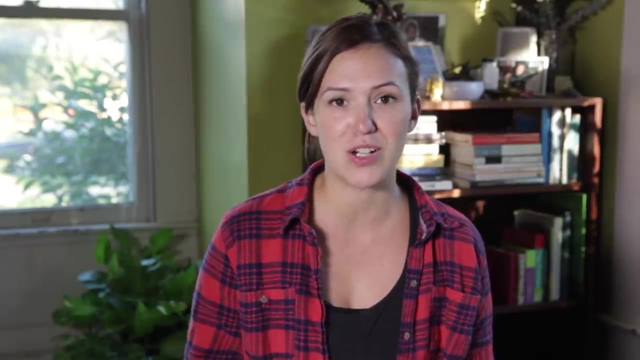 that once every day for a week and just see what happens and if you notice anything, I think you will, But who knows? All right, so those are some specifics. Try those poses in the Foundations of Yoga series. Check out the Yoga for a Complete Beginner. Part two of this: where do I start? is again. 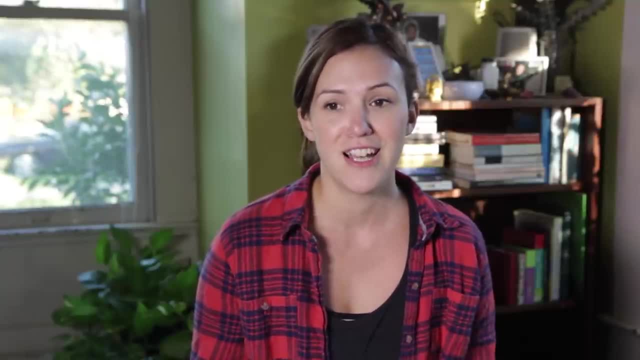 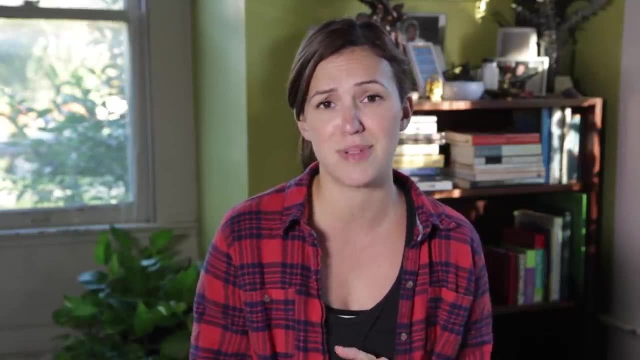 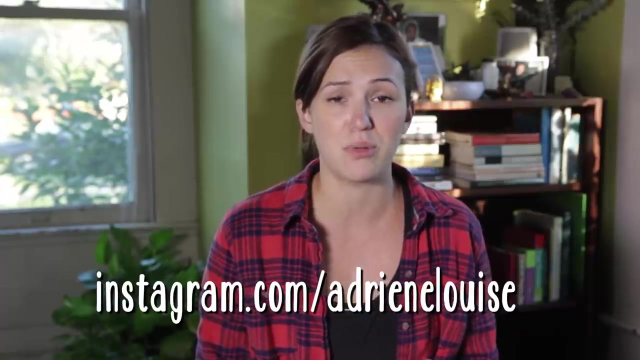 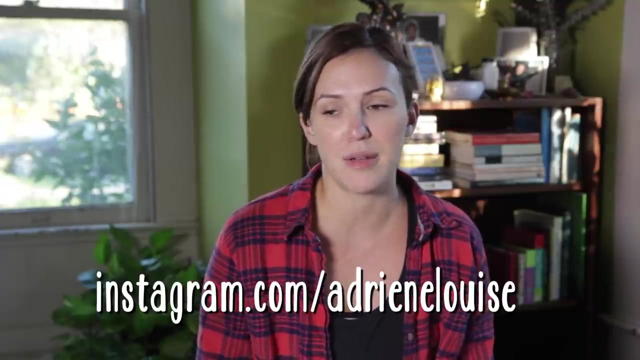 going back to here, right here, Right here, right now. get involved. Leave me questions, comments, Send in pictures if you like, Scroll through other yogis' pictures and comments and get inspired. Join the Instagram family. My name on Instagram is Adrienne Louise A-D-R-I-E-N-E-L-O-U-I-S-E, Twitter and all that. 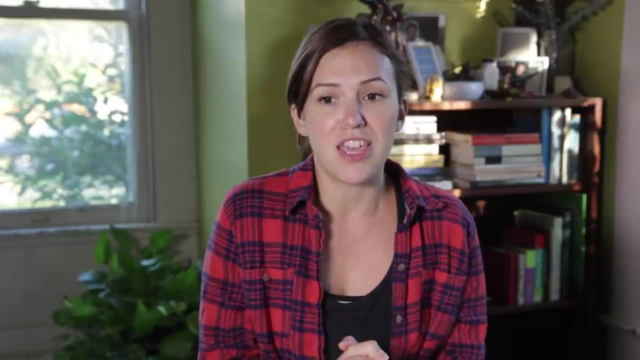 I mean, even if you're not on Twitter, so maybe that's not for you, right? The point I'm trying to make is: get involved, Help us grow this yoga. Be your own free yogi. Submit your links to the Foundations of Yoga series. 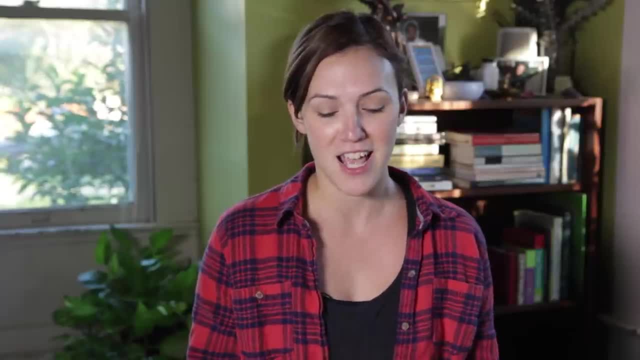 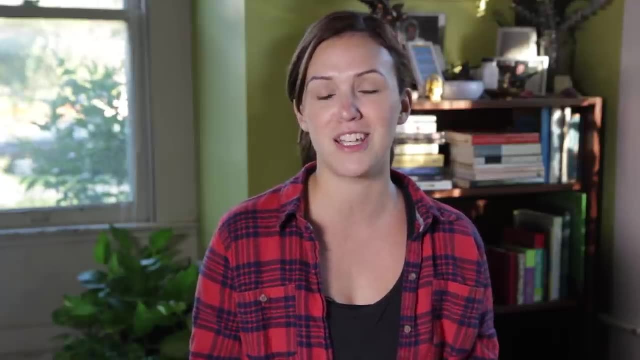 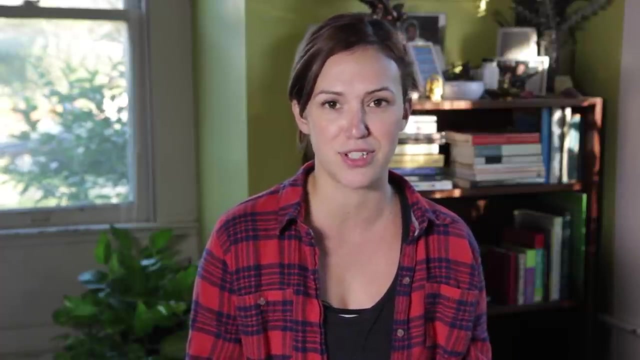 Love you, Bye, Bye, Bye, Bye, Bye, Bye, Bye. family, join us and I think you'd be surprised how actually inspiring it is. you're like: okay, I think I do want to try this today. my yoga family is doing it, Adrienne's doing it, and I think you might find a place there. it feels good. 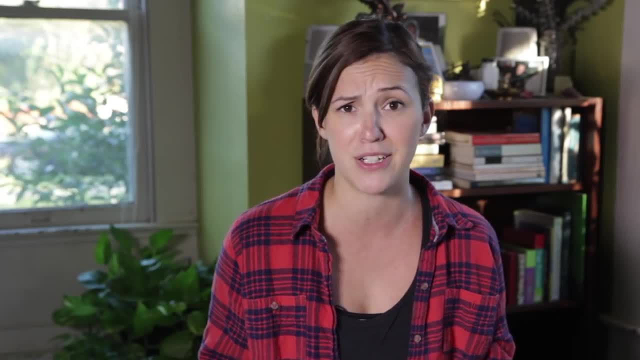 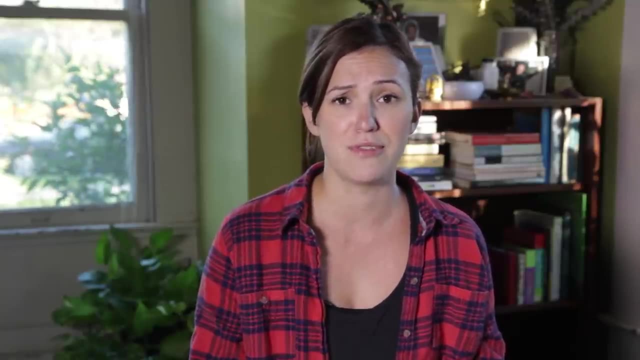 for me. I know I my life has changed ever since this channel rolled out. like I'm inspired every day- I follow my ass still every day, you know- like I learn new things every day and I'm definitely inspired by the, my fellow viewers and my fellow fellow, or Yogi's. I must went into an accent to that. all right, I think. 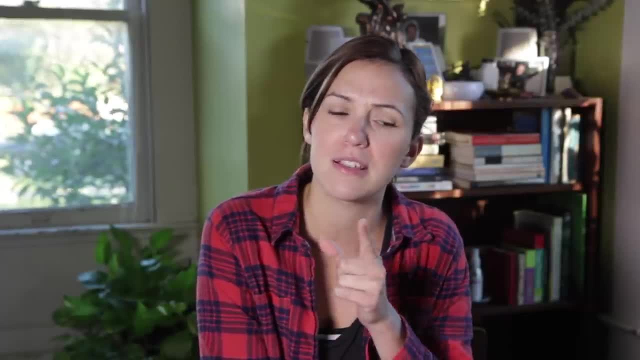 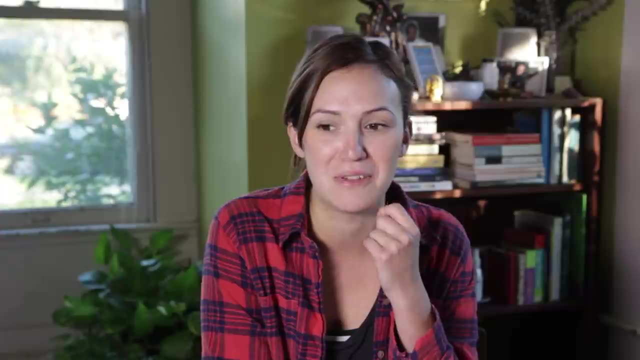 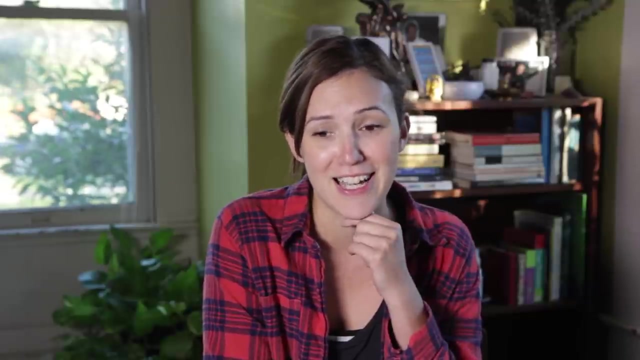 that's it for now. one other thing I could maybe put on this video is: everyone keeps asking: what kind of yoga mat do you use, and I think that might be good for beginners too. the answer is: whatever you can find that looks good and feels good for you. honestly, like I am not privileged enough. 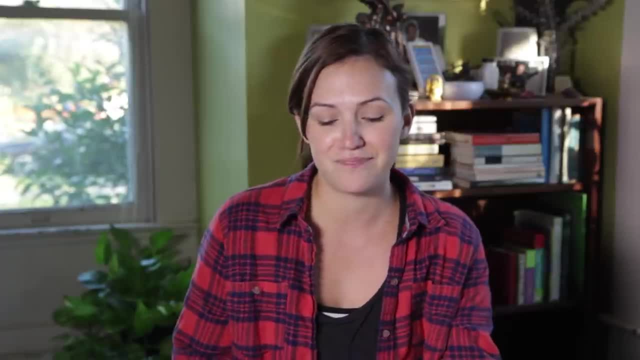 to have experienced a bunch of fancy yoga mats. maybe one of my favorite yoga mats, but I don't know, I don't know. I don't know, maybe one of my favorite yoga mats, but I don't know, I don't know. maybe one day this channel will grow and we'll all get to experience fancy yoga.